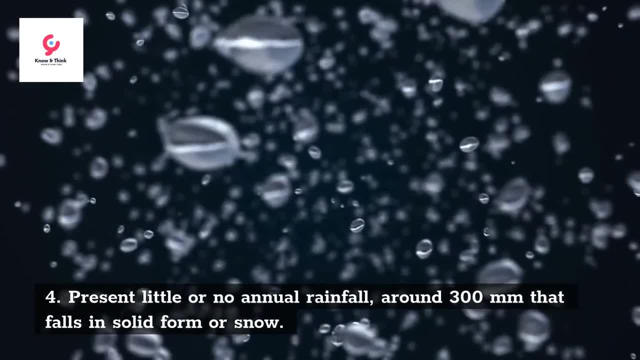 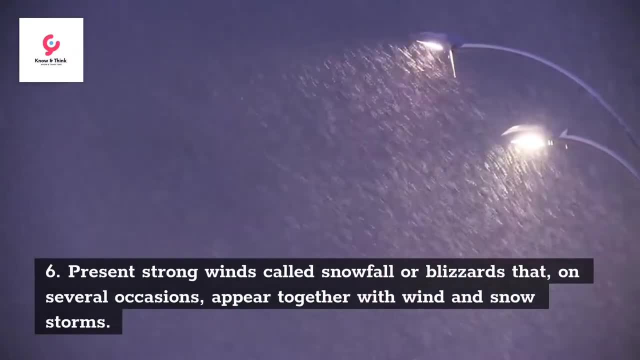 Present little or no annual rainfall around 300 mm that falls in solid form. Oregon snow. Present very little or no atmospheric humidity. Present strong winds called snowfall or blizzards, that on several occasions appear together with wind and snow storms. 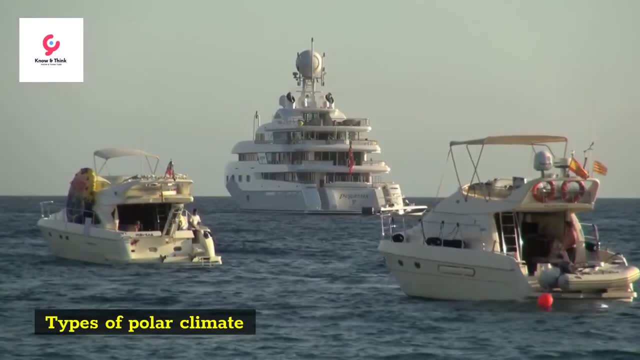 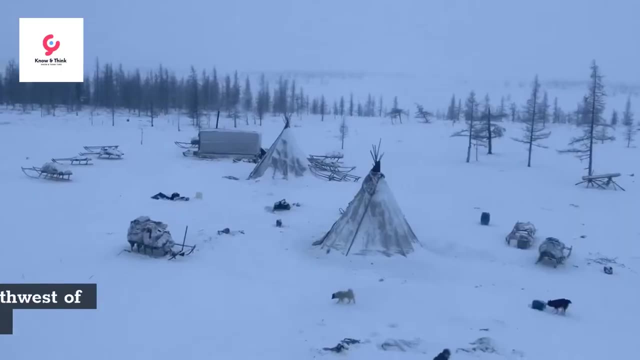 Have little fauna and flora. Types of polar climate. The polar climate. The polar climate is classified into four types: Cold, Continental. It is the climate that extends in the north and north-west of Europe, Canada, Alaska, South and Central Siberia. 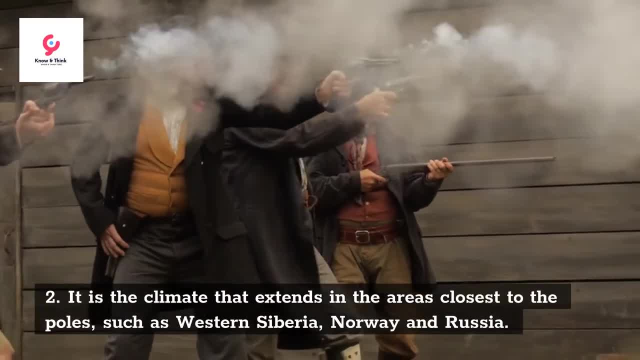 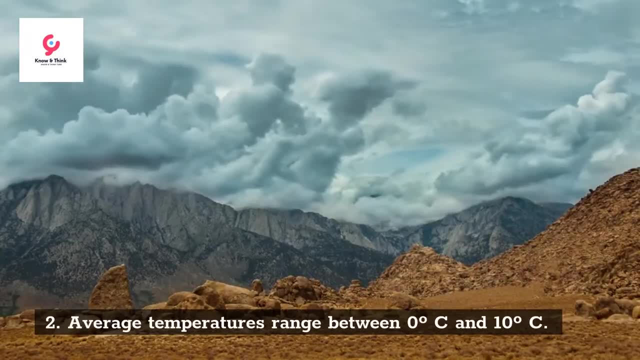 Tundra: It is the climate that extends in the areas closest to the Poles, such as Western Siberia, Norway and Russia. Average temperatures range between 0 degrees C and 10 degrees C. Polar: It is the coldest climate that extends into the areas deep in the north and south of the continent. 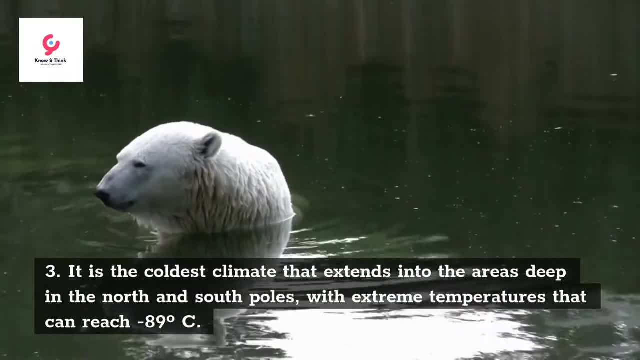 Cold Continental. It is the climate that extends in the areas closest to the poles, such as Western Siberia, Norway and Russia. So the climate that restrictionsh constructs cold climate. It is the climate that extends in the areas closest to the Poles, such as Western Siberia, Norway and Russia. 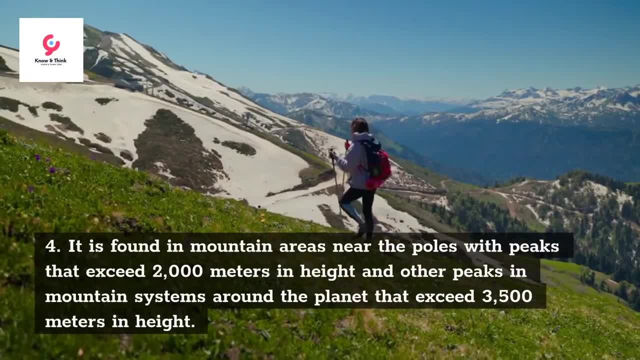 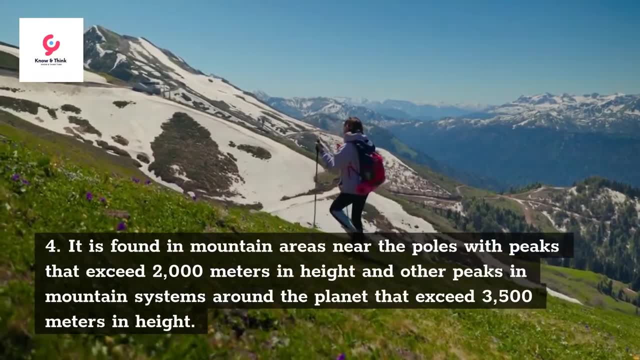 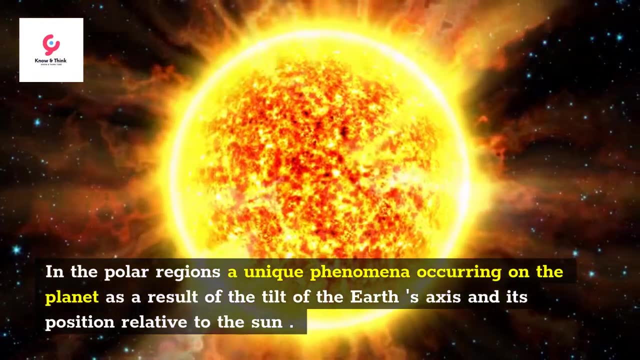 It is the climate that extends in the areasaltaight. nothing offsets its lipid wall, with extreme temperatures that can reach minus 89 degrees C. Direction of day and night In the polar regions, a unique phenomena occurring on the planet, Captain Solomai. 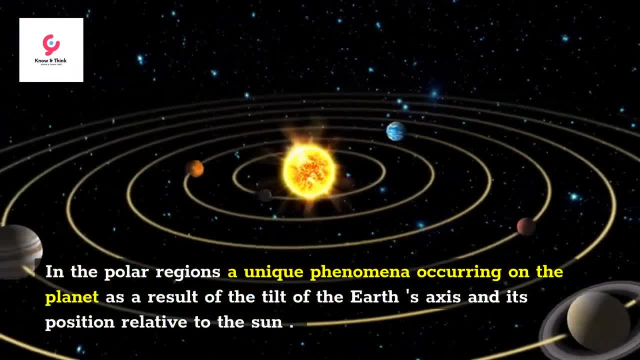 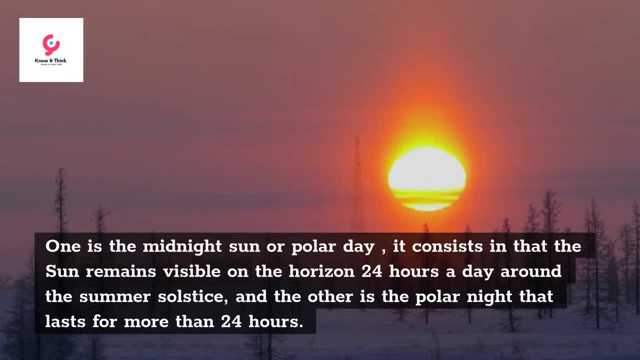 as a result of the tilt of the planet, hablando at the same space the Earth's axis and the Moon's position relative to sun In the поступing polar regone, 2000 thousand. hey asked the midnight sun or polar day? it consists in that the sun remains visible on the horizon 24. 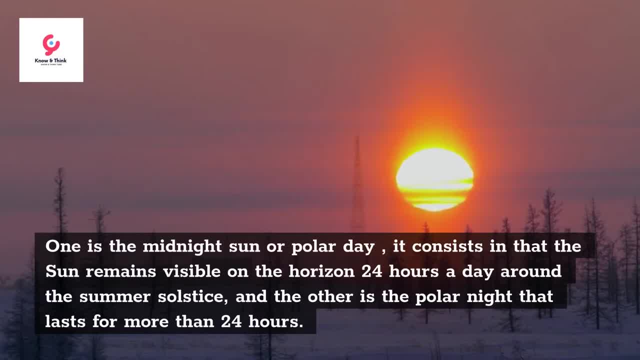 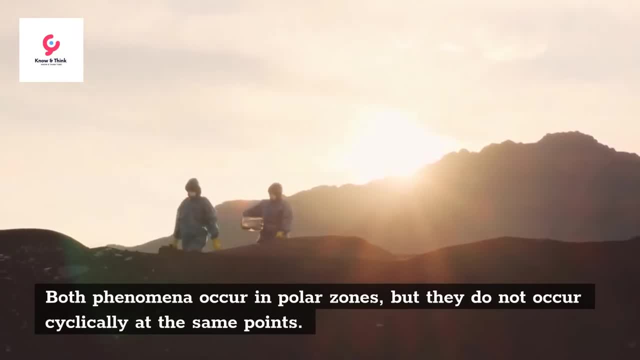 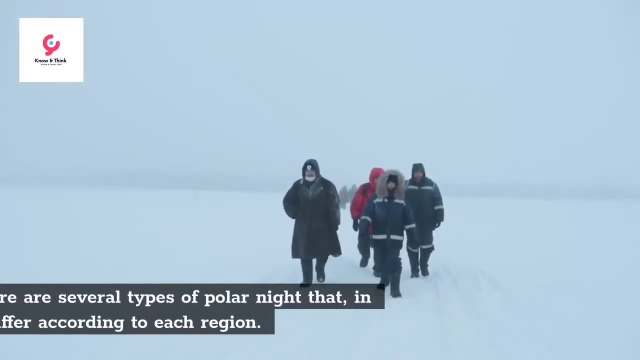 hours a day around the summer solstice, and the other is the polar night that lasts for more than 24 hours. Both phenomena occur in polar zones, but they do not occur cyclically at the same points. There are regions where you can see the polar day but not the polar night. In fact, there are 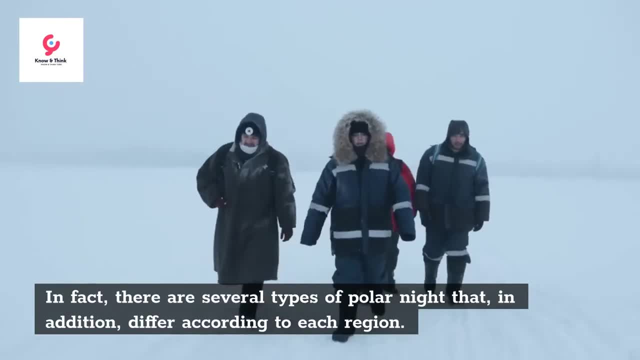 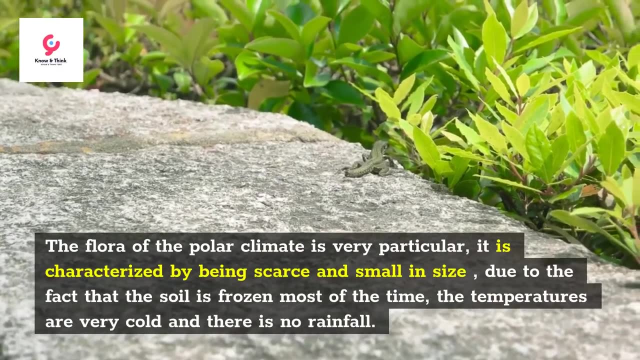 several types of polar night that, in addition, differ according to each region. Flora of the polar climate. The flora of the polar climate is very particular. it is characterized by being scarce and small in size, due to the fact that the soil is frozen most of the time. the temperatures